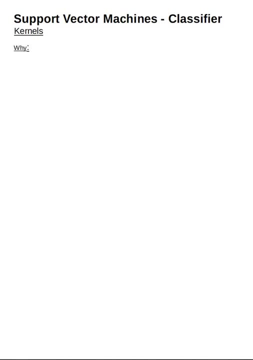 are first going to define what is a kernel. So, in the context of this video, a kernel is a mathematical function that does transformation. Typically it is a non-linear transformation. So why do we need kernels? The first question is why kernels are important to us, So for this we have to 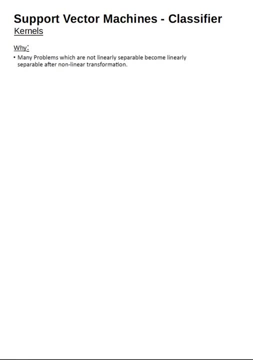 go back to some of the theorems and also some empirical observation where we can conclude that many problems which are not linearly separable, they become linearly separable after a nonlinear transformation. So this is a very important note that we have to understand. 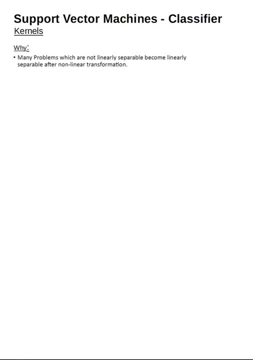 Now, one example for this is an XR problem, where in a two-dimensional space, It is not linearly separable. however, in a three-dimensional space, it is separable. Typical transformations also are transformations that will take you to a higher dimension. So that is something for us to understand: is that before transformation, we do have a particular function which is not linearly separable. 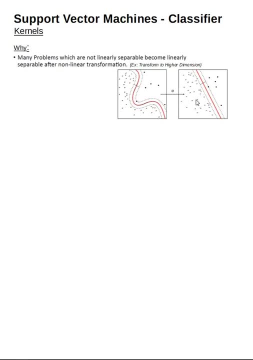 However, post-transformation, we have the same data points that now have been linearly separated. So that is an important thing to note. Now, along that note, the scheme that we are going to apply is first the input data, point xi. 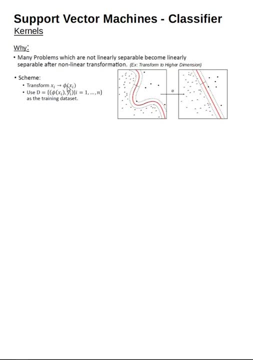 we are going to be transforming them, sending it through a phi function, a phi of xi. So therefore the overall training set becomes: d is equal to phi of xi, yi for values of i from 1 to n. Okay, that is going to become our training set. 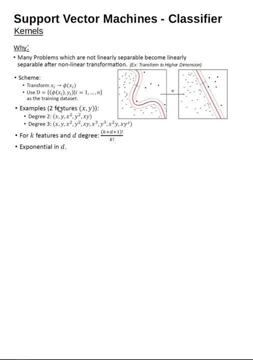 Let's look at an example. Let's say we have two features, x and y, and we want to calculate a transformation function for degree 2 polynomial. In such a case, the number of features that we will get is x, y, x squared. 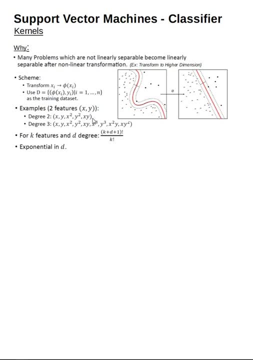 y squared and x- y. At a minimum, we could also potentially have x squared, y squared. in this particular case, In case of degree 3,, at a minimum, we are going to have not only x and y, but also we are going to have x squared, y squared, x, y, x cubed, y cubed, x squared, y, y squared, y, x, y squared, so on, so on, so on. 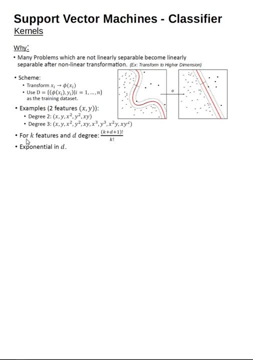 There are a lot more terms we can have, So what it means is for k features which have been input into the system. when we want to compute the higher dimensional transformation, which is what we are discussing here, as an example is, we are looking at a complexity of k plus d plus 1,. 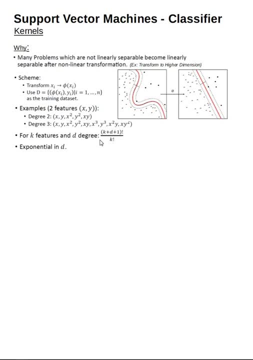 the whole factorial by k factorial. That's the complexity of the function we are looking at, That's the number of features we will actually end up having, And this feature list is actually going to be growing exponential to d, which is the dimension, which is the degree with which we are. 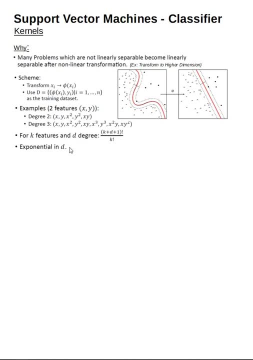 currently expanding. okay, So that's the key note for us to understand, And what we have to know is that, now that we know that, if we were to take data to a higher dimension, and having taken the data to a higher dimension, 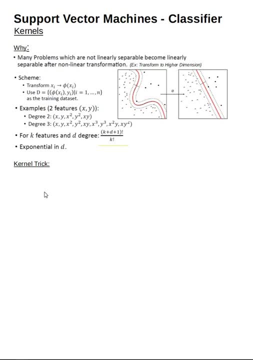 how do we now apply it into our existing support vector machine mathematical space? Okay, So that's where the concept of kernel tricks come in. So one thing to note is that we spend time understanding the dual formulation in the earlier lectures, because the kernel trick actually operates only on the dual formulation. 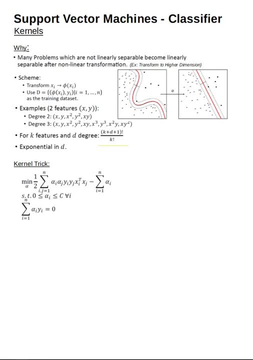 and not on the primal formulation. okay, So that's an important thing to know. Next important thing to know is, after we have done a transformation of this kernel, with the kernel function for our standard dual formulation, which is given in the left-hand side. 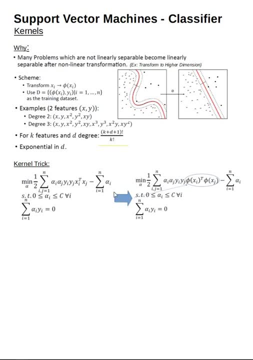 so if we see the dual formulation, it is the dual formulation that we had already derived for our SVM. So minimization of half sigma sum of alpha i, alpha j, y, i, y, j, x. transpose i, x, j minus the sum of alpha i. 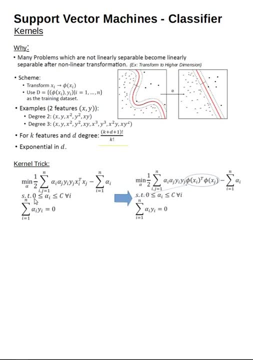 And they were constrained to zero and the alpha i's were constrained between zero and c And this is the soft margin, SVM, dual formulation, Okay, That we had derived. Now, when we do a change- mathematical notation change- what we are doing is: 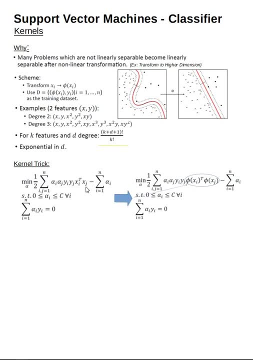 we are directly embedding the kernel transformation. In place of x, i transpose x, j, we are putting it: phi of x, i transpose into phi of x j. Okay, That's the first thing we are doing, And one very neat thing that gets called as a kernel trick. 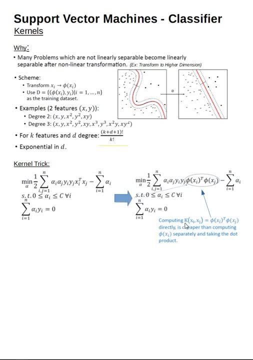 is that when we do a computation, for example a kernel function, k, x, i, x, j- which is nothing, but in this current case is phi of x, i transpose x, j- we can do a direct computation of this value and that direct computation is cheaper than computing separately. 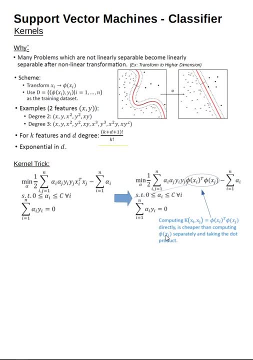 a kernel value of phi of x- i and separate value for phi of x- j and then taking a dot product. Okay, So this particular notion that we can directly compute this value instead of separately computing them and taking a dot product. 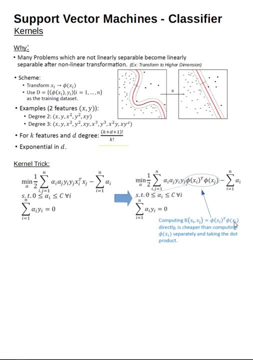 saves us the computational complexity, and it gets called as the kernel trick. Okay, So now let's look at what sort of a training logic- overall training logic- then becomes. So, first things, what gets to happen is we are given a training data set, D. 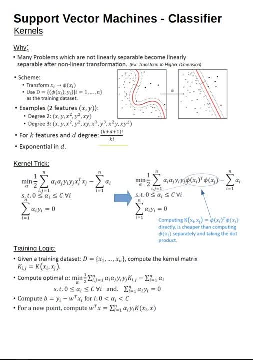 with x 1 to x n in data, and now we compute the kernel matrix. So kernel matrix is k i, j, which is computed as the kernel function of x, i, x, j. Okay, For this given data set. Next, what we are going to do is: 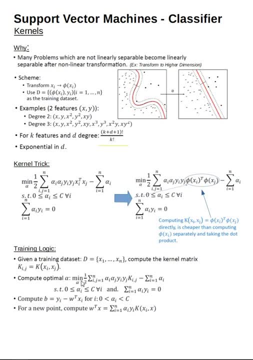 we are going to compute the optimal alpha, which is nothing but gradient descent or a related optimization algorithm that we will apply onto this minimization function for us to get our optimal alpha. And note here we have replaced it with k i, j. 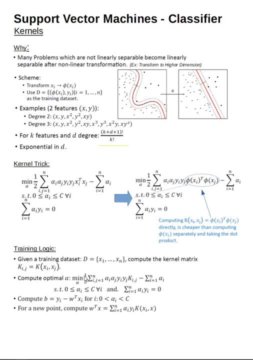 and not x, i, x, j. Okay, So from this particular optimization perspective, it is running directly on the kernel functions. Next we compute the b. having computed the alphas, we have enough information for us to be able to compute b. 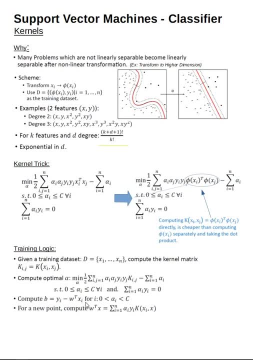 to be y, i minus w. transpose x for each value of i, which is currently bound between 0 and c, because the alpha values are bound between this. Okay, Now, if a new value comes in in a particular case, let's say: this is how far we'll do. 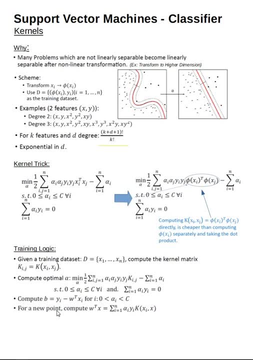 till the training data is concerned, but post this in the test when the test data is passed over, which is what we are writing. as for a new point that's coming in, we compute w, transpose x, which is the new point's value. 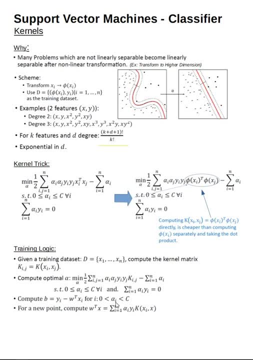 as is equal to the sum of i, 1 to n, alpha, i, y, i for the kernel value, where we are passing in x, i comma x, which is our new training data set point. Okay, So that's what we do Now. 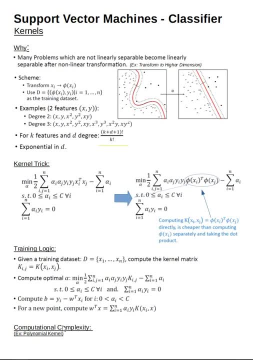 that's the overall training logic. Now let's look at a very quick example of how computational complexity is reduced. Remember earlier we saw for a k-featured data set with d degrees of computation. we were growing exponential in d, but now we are actually going to be growing. 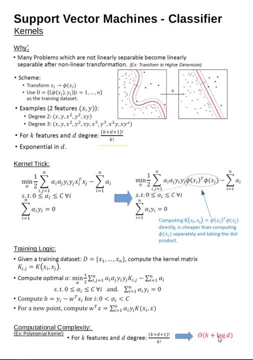 our computational complexity is in the order of k plus log d, So we are now growing in the space of log d and not exponential d, which is a significant computational complexity reduction because of this kernel trick. Okay, So that's all for this video. 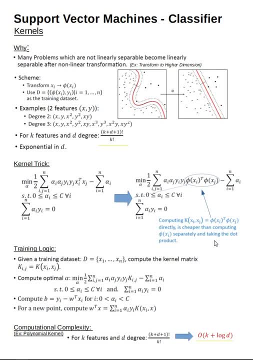 I hope you guys enjoyed it. The subsequent videos I'll cover the kernel types and also we'll discuss how to build new kernels and what defines mathematics and what defines mathematically as a kernel. In the current video we simplify the definition of a kernel as any transformation function. 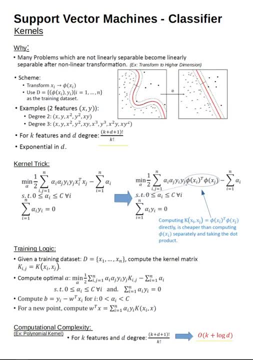 However, in the subsequent videos we will mathematically put the necessary framework around what defines a kernel. Okay, All right, I'll see you guys in the next video, Thank you.